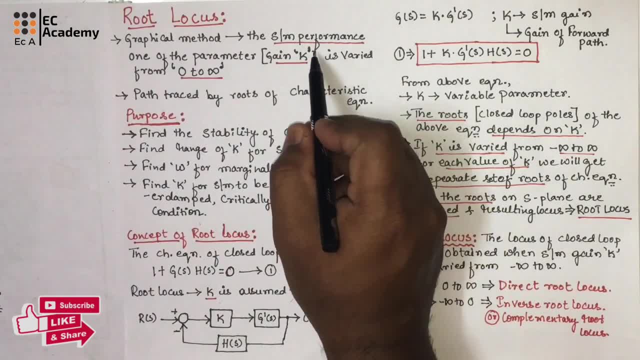 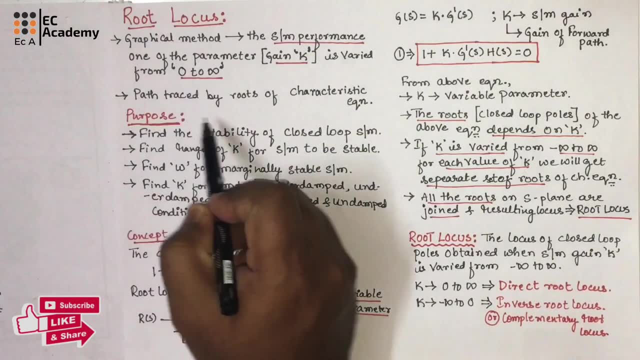 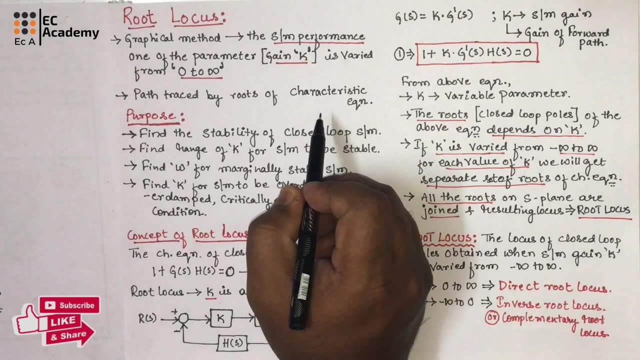 from 0 to infinity. So which means in a system, k will act as the variable. Root locus is the path traced by the root of the characteristics equation. So when we find the root of the characteristics equation, that will define the stability of the system. 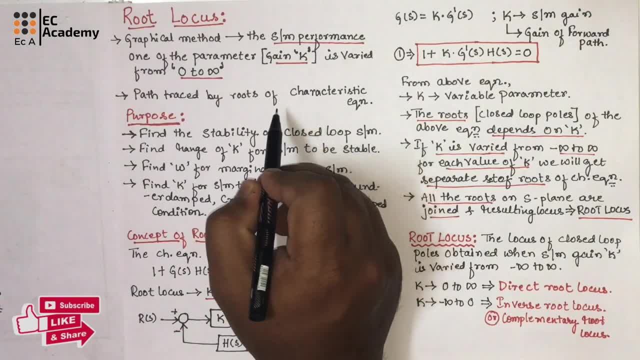 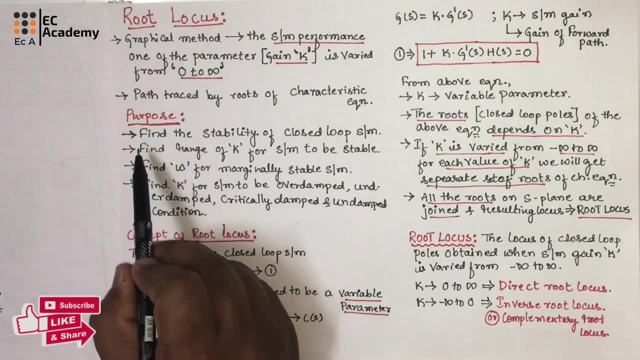 When we trace the path of the roots. that locus is known as root locus. Now let us understand the purpose of root locus. Root locus is used to find the stability of the closed loop system. To find the stability of a closed loop system. 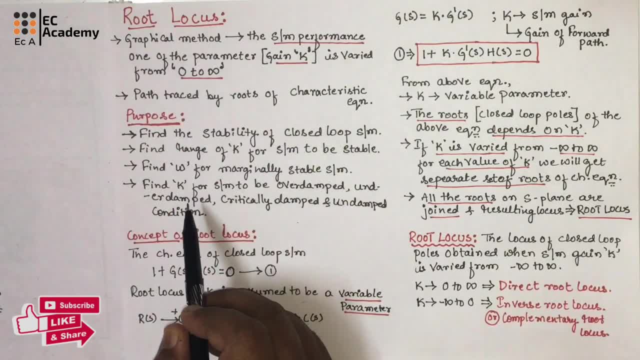 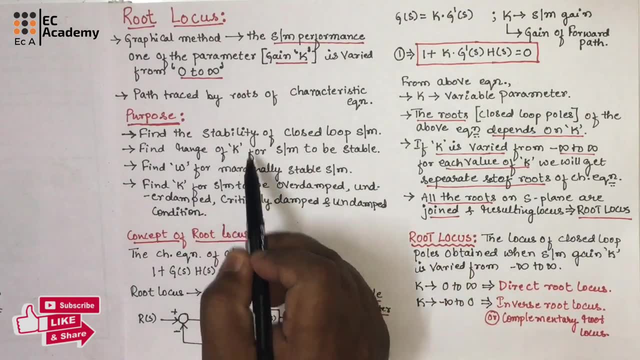 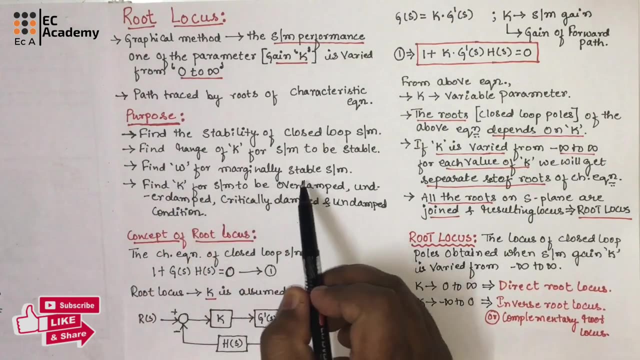 we will go with a graphical method, which is root locus. It is used to find the range of k for system to be stable, So we will find the value of k for which the system is stable. Also, we will find omega for marginally stable system. The frequency omega is found to find if system is. 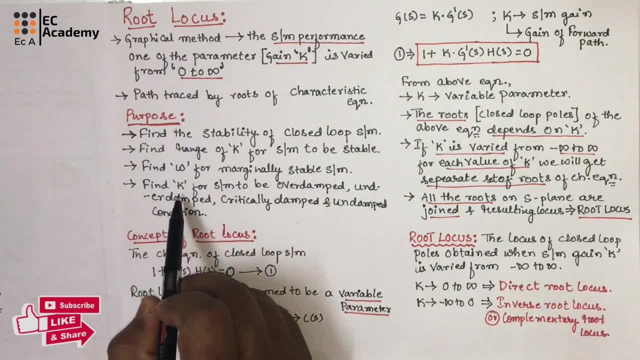 marginally stable or not, We will find the value of k for system to be over, damped, under damped, critically damped and undamped conditions. So to analyze different conditions of the system, we will find the value of k using root locus. Now let us understand the basic concept of root locus. 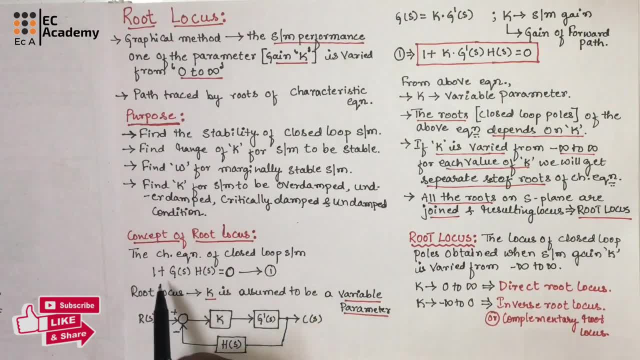 Let us take the characteristics equation of the closed loop system that is given as 1 plus G of s into h of s is equal to 0.. Let us take this as equation number 1.. In case of root locus, k is assumed to be variable parameter, so always we want to get root locus. So root locus equals to입 element. System of C腾 benefit am kingp cshaped of chp and przymf ofG. that is a required condition. So in previous video K is assumed to be multiple variable parameters. So 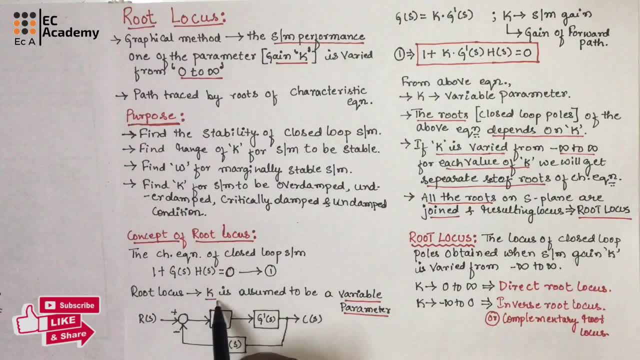 is agreed that k would be a variable parameter. So always你知道 that wh would be a variable because we want to get T of s step這個 premise of log for the system, So parameter. So always k is assumed as a variable parameter in case of root locus, which means we: 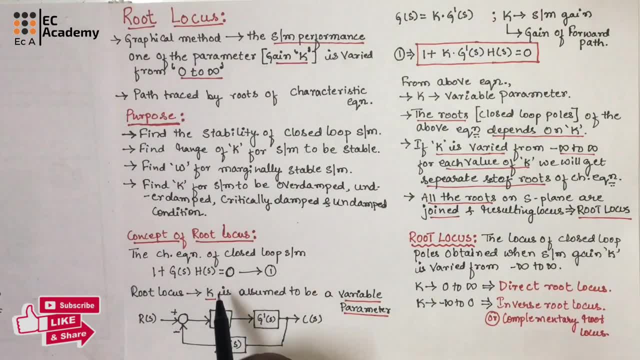 will vary the value of k from 0 to infinity to find the system performance. That is why we will take k as variable parameter. Let us consider a closed loop system. In this closed loop system, let us take g of s as k into g dash of s, So we can write g of s is equal to k into 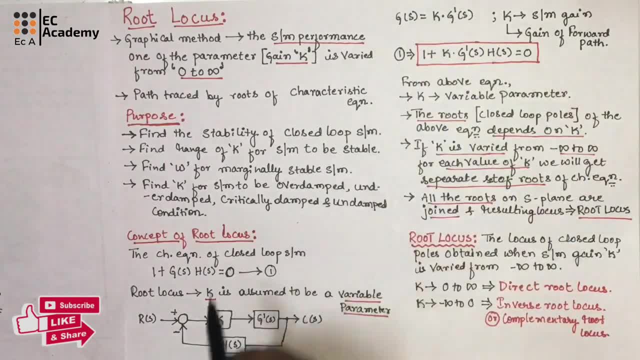 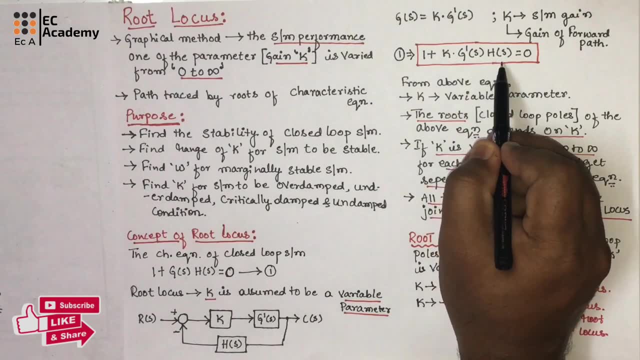 g dash of s. So if we substitute this value in equation 1, we will get 1 plus k into g dash of s, into h of s is equal to 0. So this will be the characteristics equation. Here k is the system. 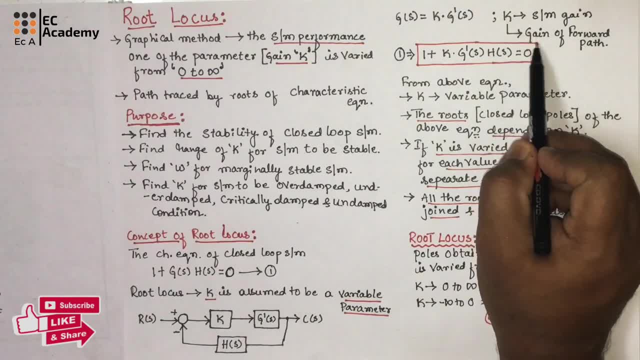 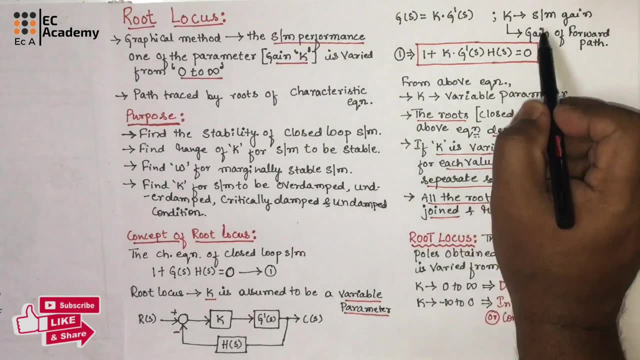 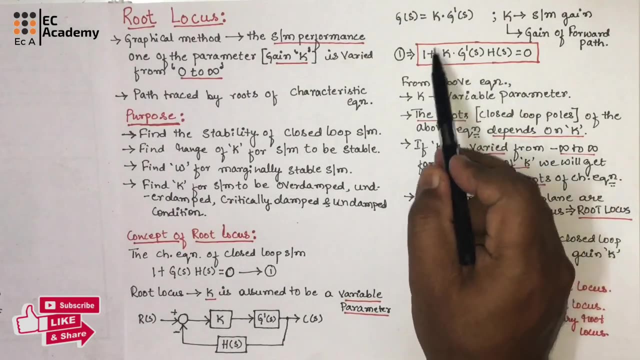 gain, and it is also known as gain, Gain of forward path. So in this closed loop system k will act as gain of forward path or it is the overall system gain. From the above equation we can say that k is the variable. 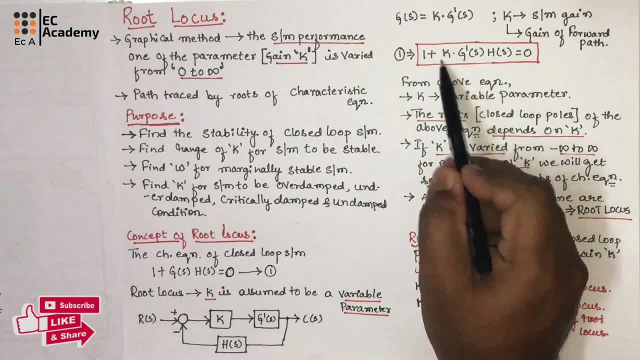 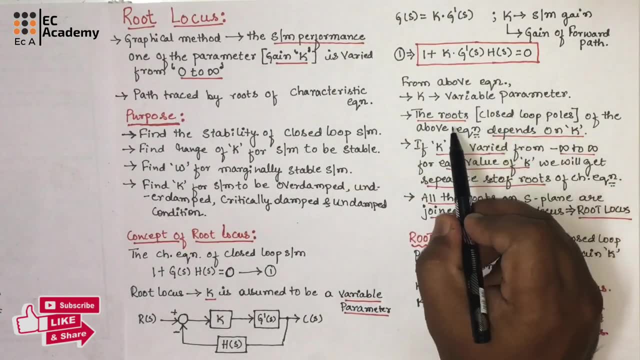 parameter. So here k will act as variable parameter. The roots of the above equation depends upon the value of k, So the roots, which is also known as the closed loop poles- of the closed loop system. So in this closed loop system we can say that k is the variable. 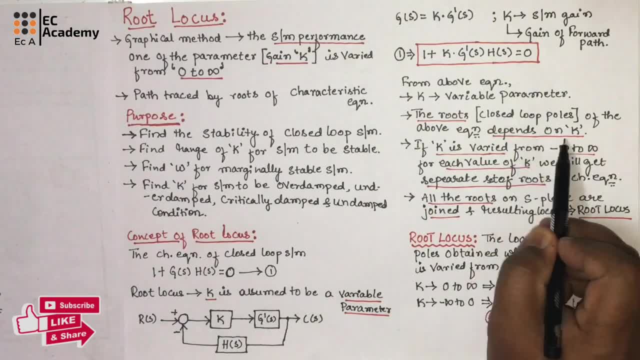 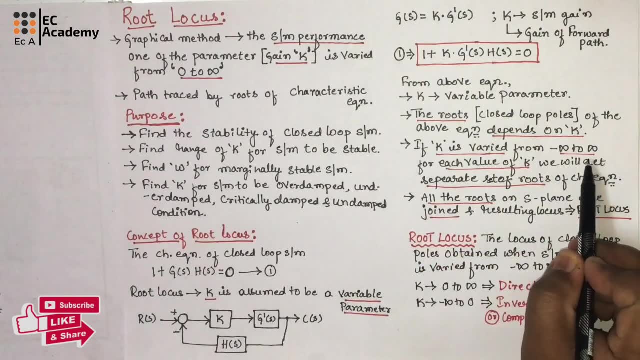 parameter. So in this closed loop system we can say that k is the variable parameter. So the characteristics equation will depend upon the value of k. In this equation, k is varied from minus infinity to infinity. and for each value of k, from minus infinity to infinity, we will get 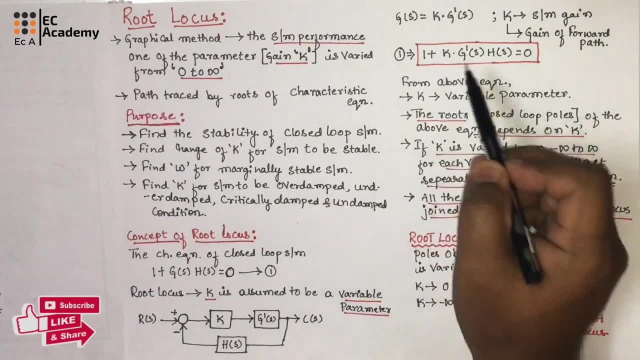 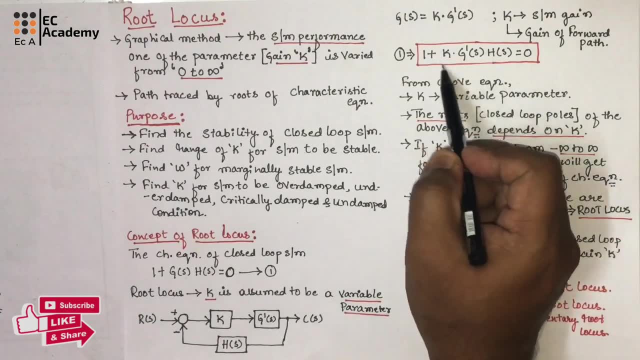 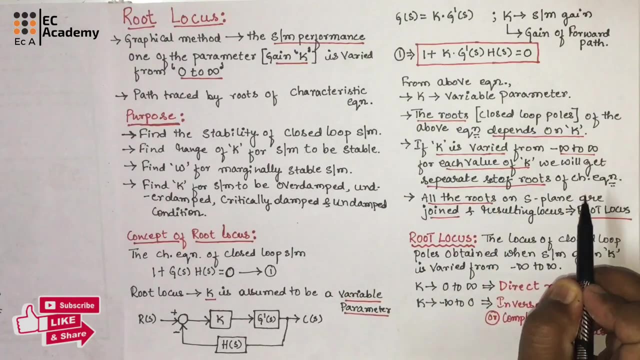 separate set of roots. For each value of k we will get different set of roots for the characteristics equation. So here we need to vary the value of k from minus infinity to infinity, and for each value of k we will get separate set of roots of the characteristics equation. If all the roots on 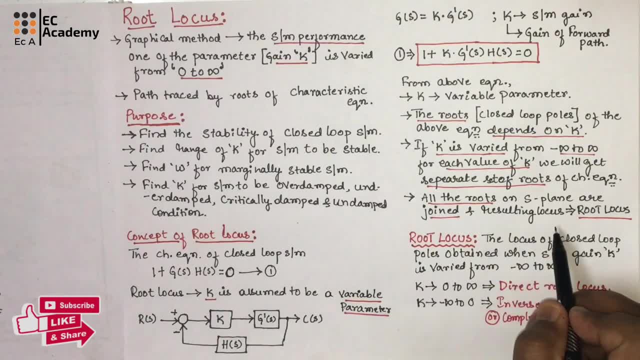 s plane are joined, and the resulting locus is known as root locus. Once we find the roots of the characteristics equation, if we join all these roots on the s plane, the resulting locus is known as root locus. So we can define root locus as the locus of closed loop poles obtained. 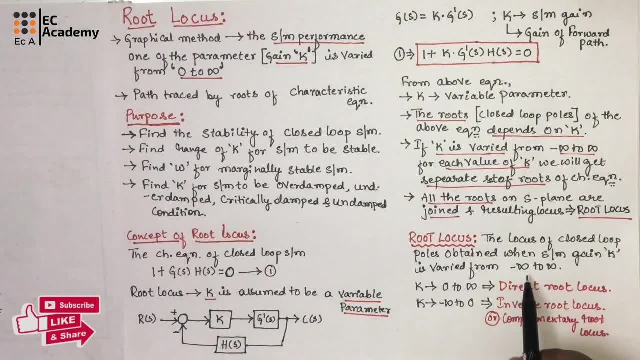 the system gain, k is varied from minus infinity to infinity. So it is a locus of closed loop poles which is obtained when the value of k is varied from minus infinity to infinity. Now, when the value of k is varied from 0 to infinity, the plot is known as direct root locus. Usually, we will be. 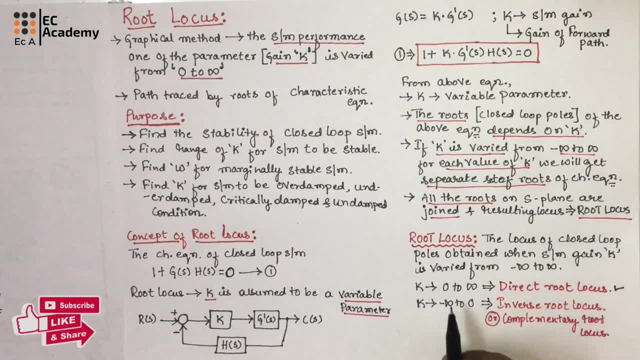 finding this root locus in our examples where we will vary the value of k from 0 to infinity. If we vary the value from 0 to infinity, the plot is known as direct root locus. If we vary the value of k from minus infinity to infinity, we will call that as inverse root locus, or complementary. 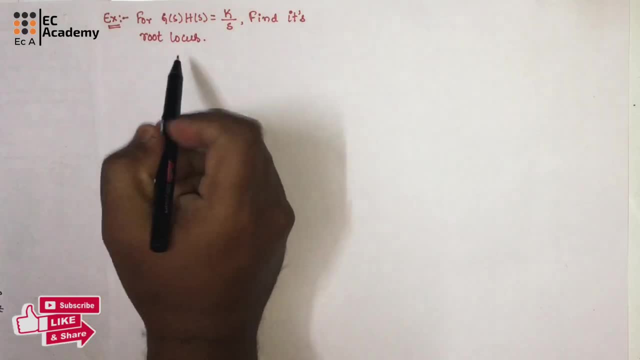 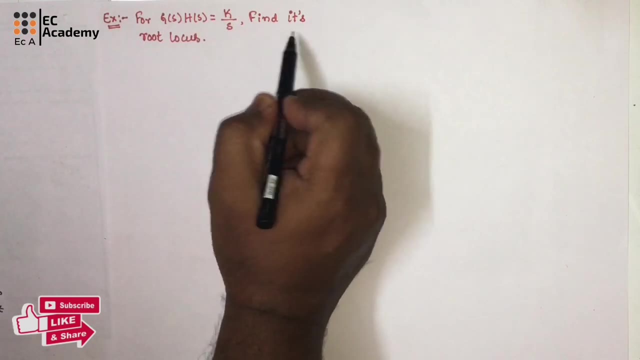 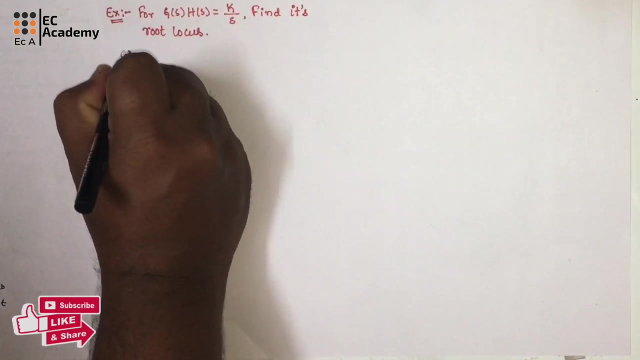 root locus. To understand the concept of root locus, let us take an example where g of s and h of s is given. For this we need to plot the root locus. First. let us write the characteristics equation. We know the characteristics equation can be given as: 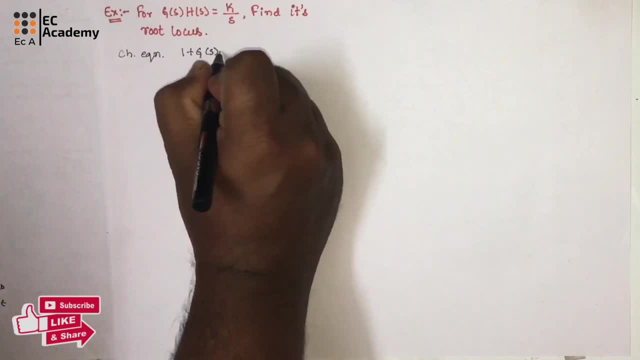 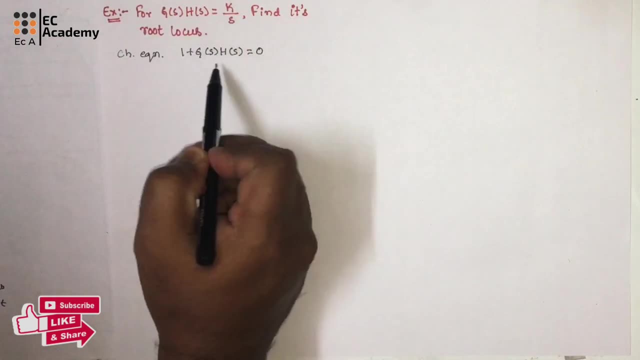 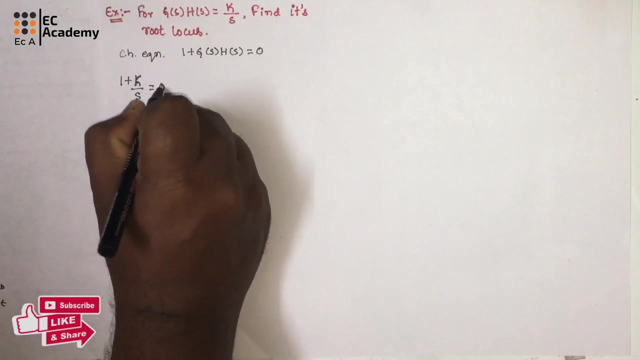 1 plus g of s into h of s is equal to 0.. Now g of s into h of s is given. Let us substitute in this equation: We will get: 1 plus k divided by s is equal to 0. So from this we can write s plus k. 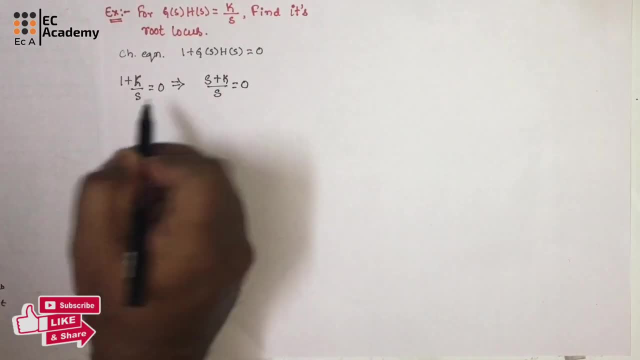 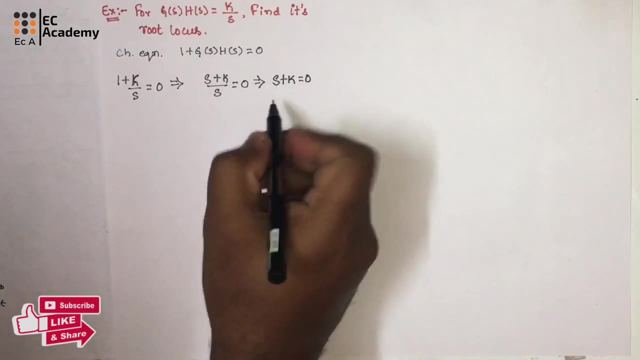 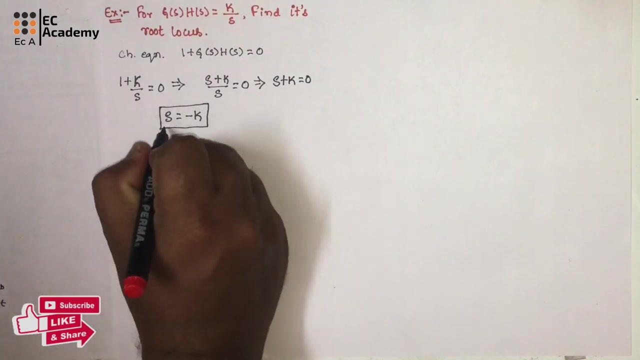 is equal to 0. We have taken the LCM here. From this equation we can write s plus k is equal to 0. So we can write: s is equal to minus k. In this equation s represents the root and k is the. 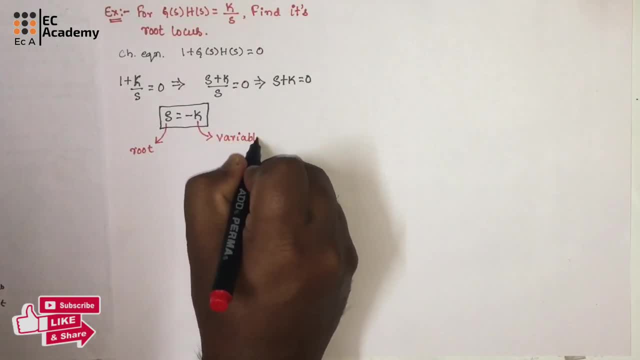 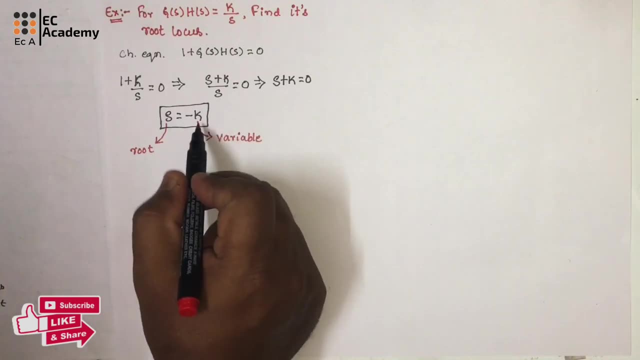 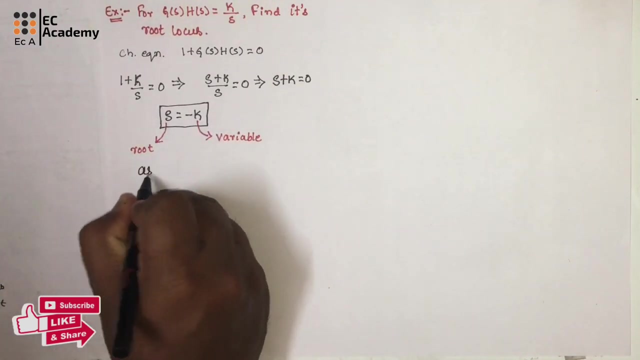 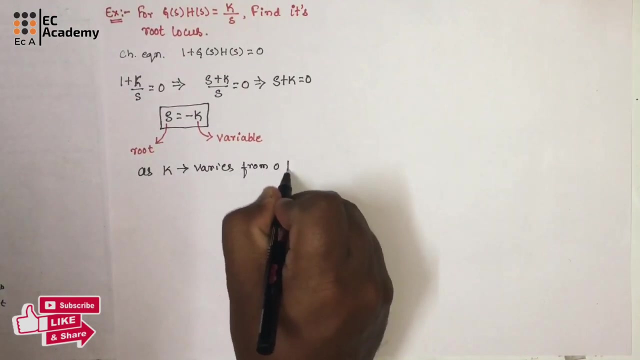 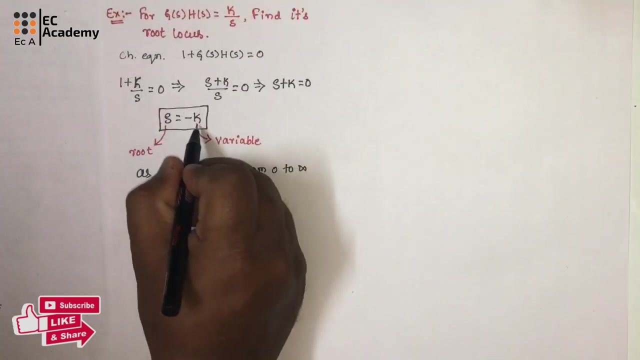 variable. So we can say the roots of the k가�. adesso�이 characteristics equation is depending upon the variable k. So as we vary, the value of k, s will also vary. As k varies from 0 to infinity, the value of s also varies. Now let us take k. 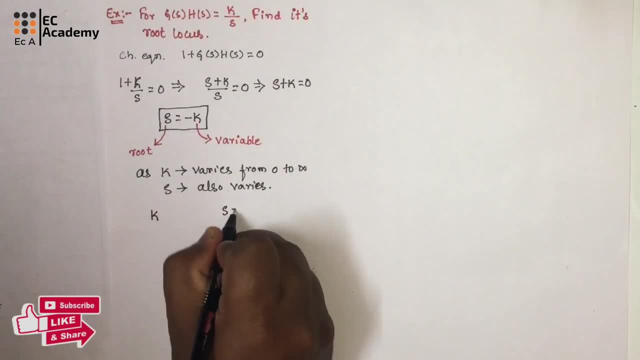 and s, which is equal to minus k. Now let us vary the value of k from 0 to infinity. When k is equal to 0, s will be equal to 0.. When k is equal to 1, s is equal to minus 1..